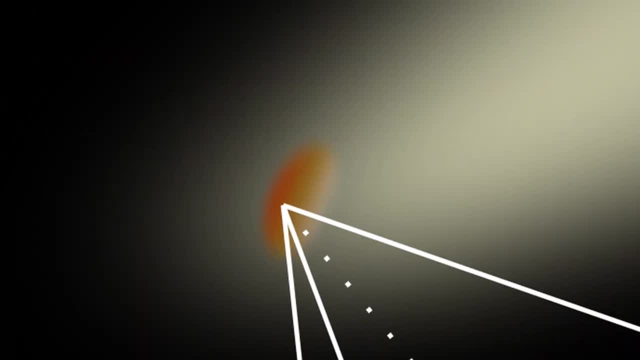 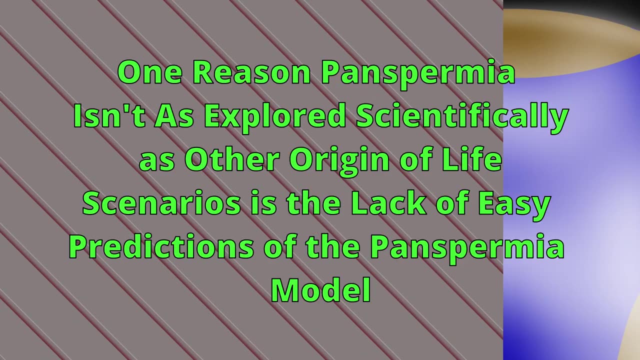 difficult to rule out. And because it's difficult to rule out this idea that life came from somewhere else, it sets a lot of scientists at edge, and scientists are particularly weary of ideas like this. Scientists tend to like predictions and to an extent, these blind-sense ideas don't lead to. 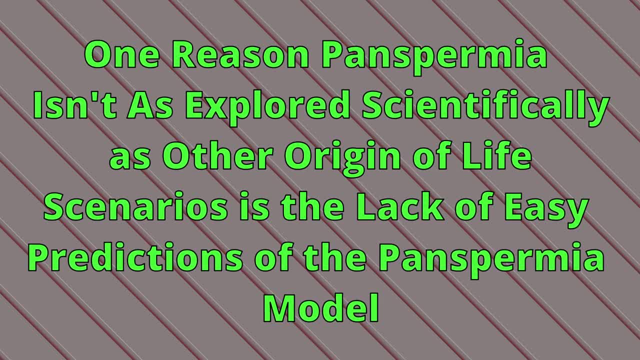 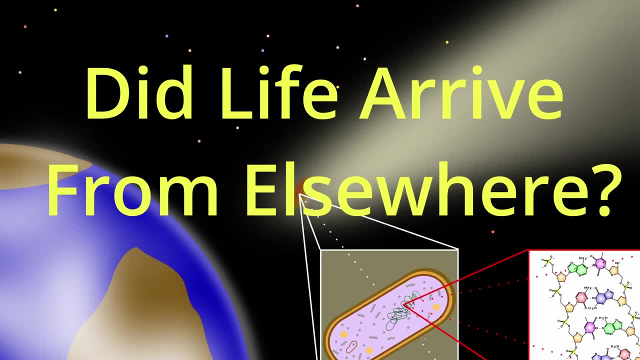 easy predictions. That is, to an extent they don't consider ideas because they don't readily lend themselves to easy predictions. But nonetheless, when considering this broader conversation of the origins of life, as we're starting it now, we have to consider the possibility. 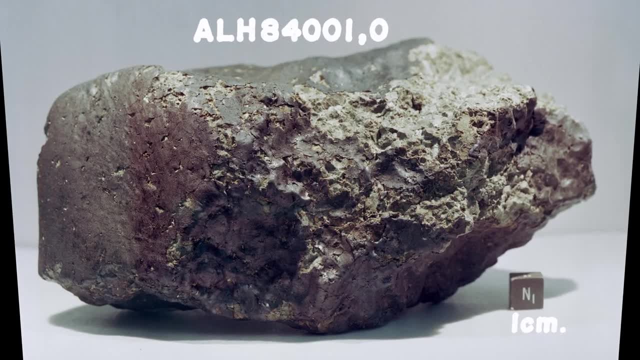 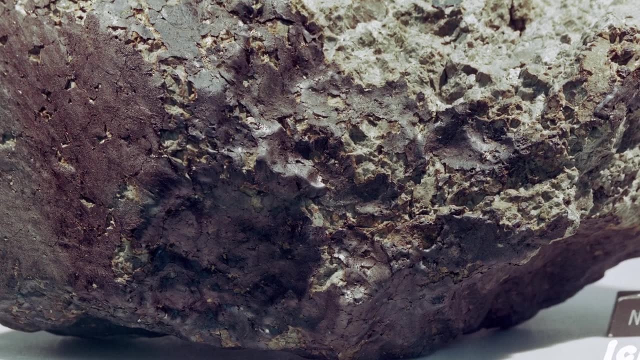 of life elsewhere. To that end, we're going to turn to Alan Hill's 84001, which, with all the controversy around it, has yet to be entirely laid aside as possible evidence of life on Mars. Alan Hill's 84001,: it's a meteorite. 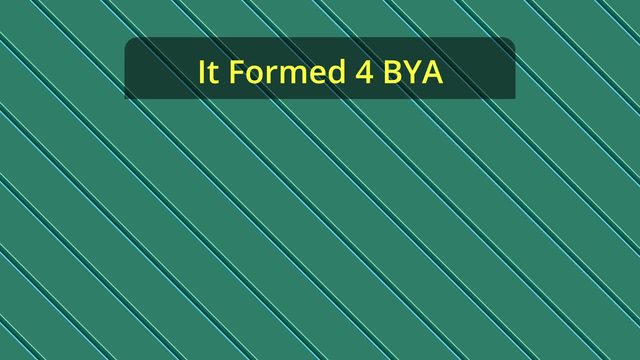 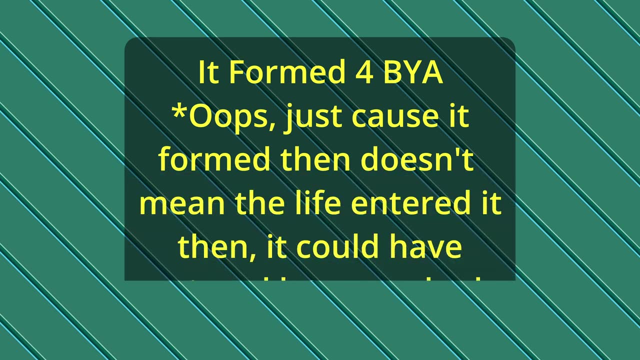 which is very likely to die from Mars. Radiometric dating of the meteorite indicates an age of about 4 billion years old, which is older than any widely accepted evidence for life on Earth. so this would be older than any known life on Earth Four billion years ago. 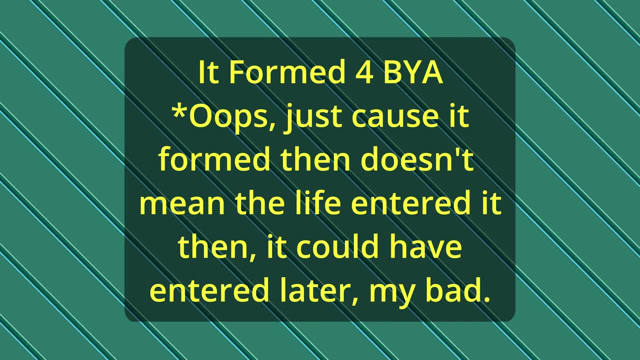 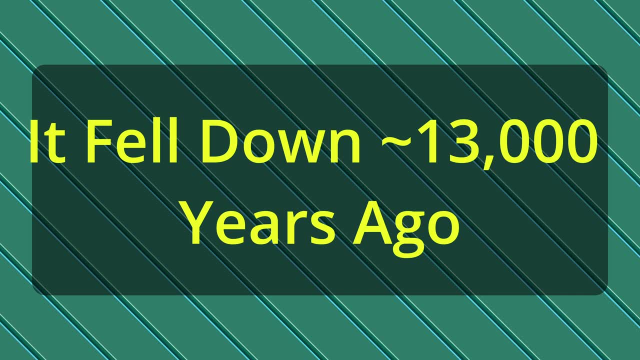 this rock was born through igneous processes and more recently, 50 million years ago, it's knocked off Mars and flung out into space, where it chilled for a while before getting caught in Earth's orbit and crashing home in Antarctica. 84001 was first picked up in 1925,. 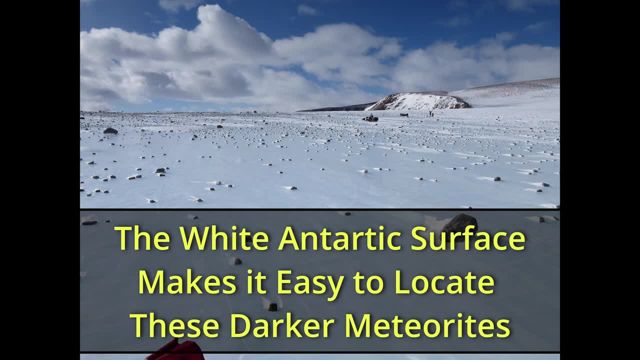 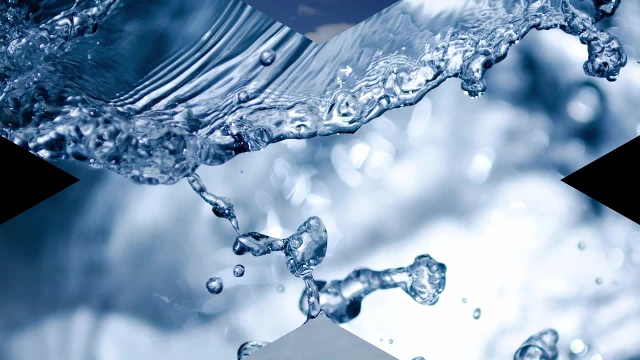 1984, and it was immediately recognizable as very different from the other meteorites. For one, it had minerals that suggested the possibility that it had interacted with liquid water. If it had interacted with liquid water, this would be evidence that Mars had water. 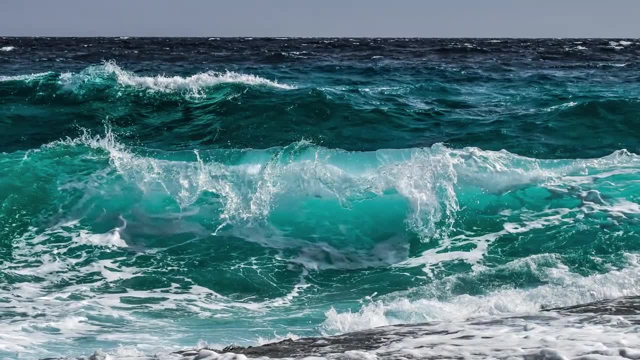 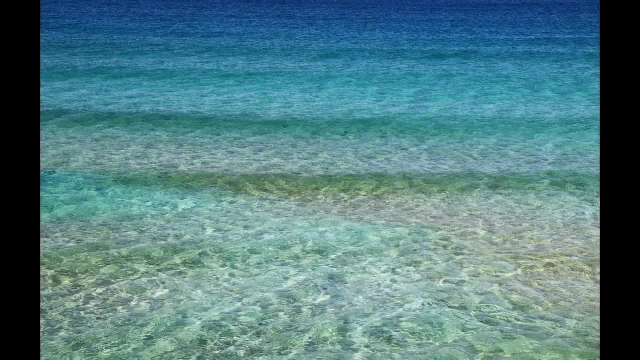 Of course, now we know that Mars had abundant water, but at the time the pursuit of this question was incredibly important, and because of that, NASA set a team upon it to analyze it intensively, possibly more intensively than any rock had ever been studied prior. 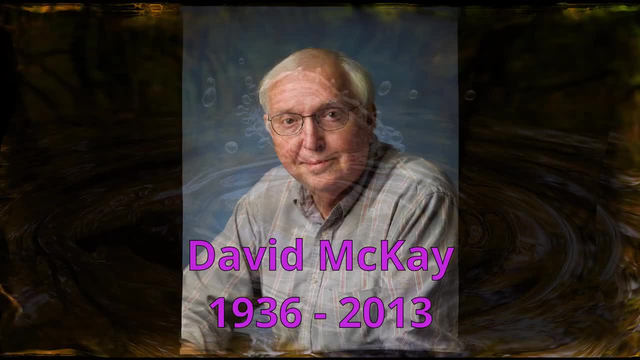 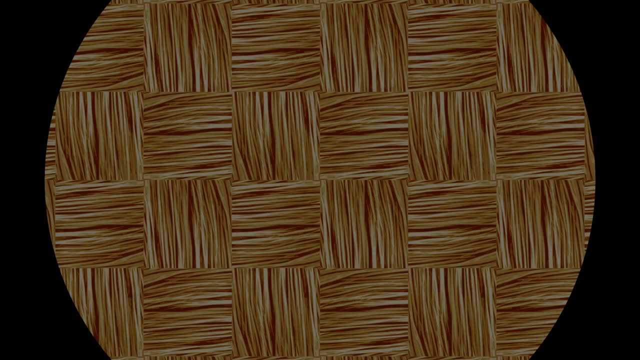 in the history of the universe or our planet anyway. This NASA scientist group was led by David McKay and they came around in 1996 to announce that they think they found evidence of life in it. There are a number of lines of evidence that they mention in their paper, and here's what. 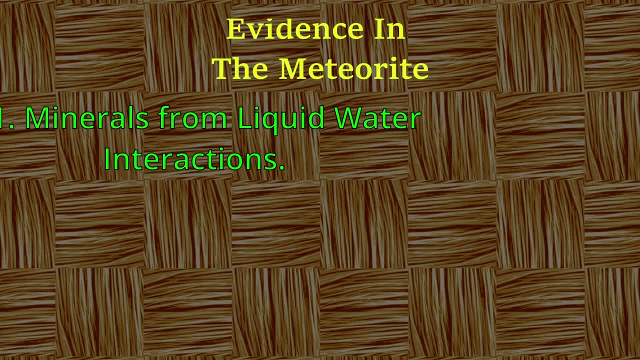 the overwhelming majority of the evidence was One: they showed evidence of liquid interactions leaving behind specific minerals, and that shows that something that's often thought to be a necessary condition for life- water- existed on Mars. Second, they showed a compound called a polysaccharide. 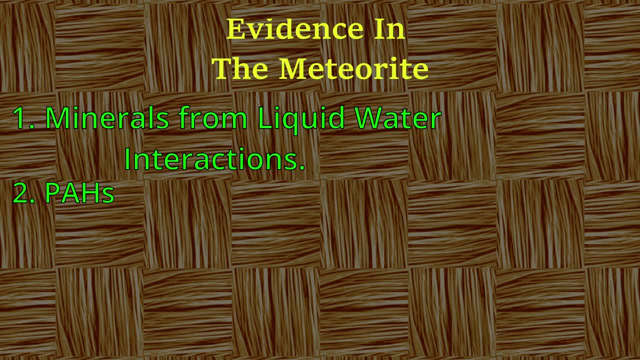 Polycyclic aromatic hydrocarbon, or a PAH. PAHs are small carbon-based molecules that remain long after a bacteria has died. They often come about when a once-living cell is exposed to a high temperature and, because they're particularly sturdy, they don't get destroyed and they can survive for a long. 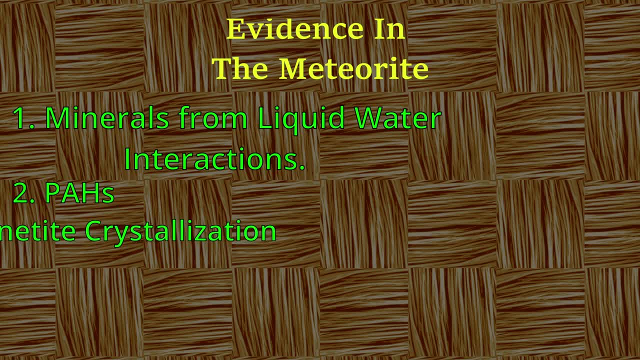 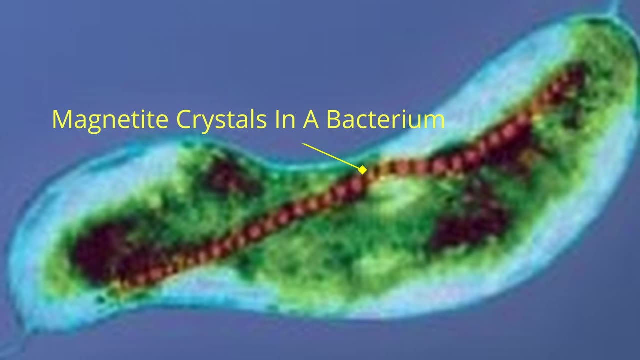 time We could find them eventually. So we have these PAHs in this meteorite. Third, they showed that certain iron-bearing minerals, specifically magnetites, appeared that they're not known to appear in nature And in fact the only place that at the time we knew it could appear this way are in a 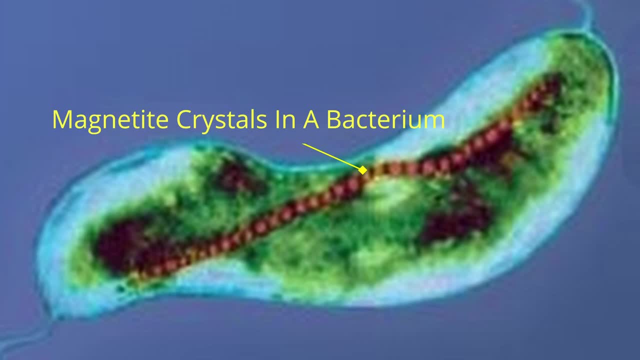 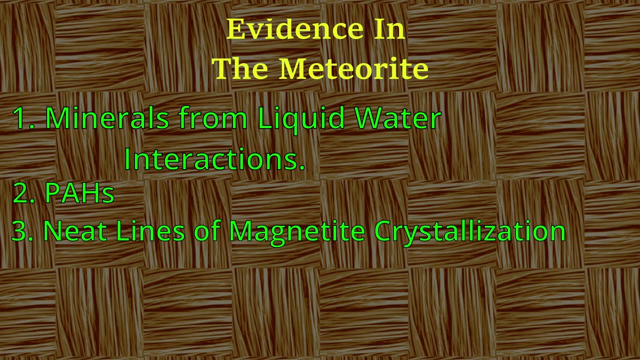 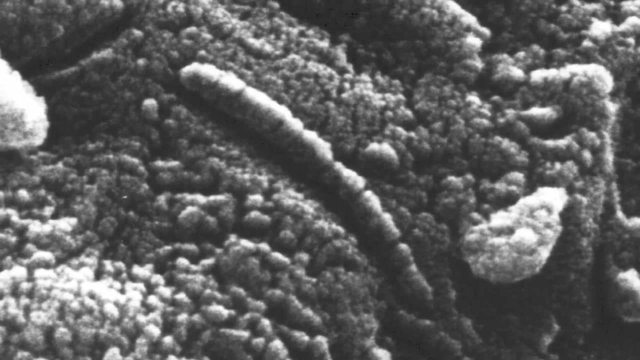 certain type of bacteria, magnetotatic bacteria, And these bacteria produce these magnets in this nice neat line and use it as a magnet to know up from down, based off of the Earth's magnetic field. And lastly, there are these tiny 20 to 30 nanometer elongated sausage shapes that were 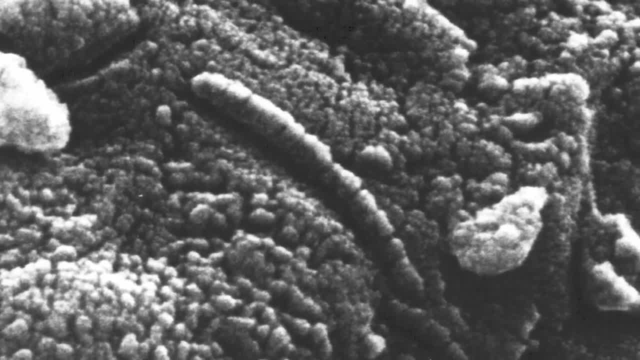 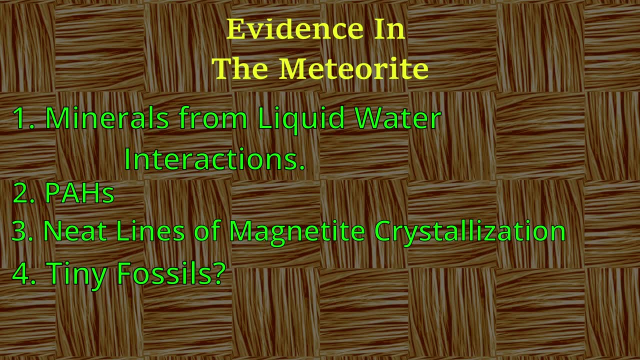 found and they looked like they just might be fossil microbes, Although these fossil microbes would be on a scale significantly lower than any known life on Earth. So just to review the four lines of evidence: One: there's evidence of water based off some minerals that seem to have been created through 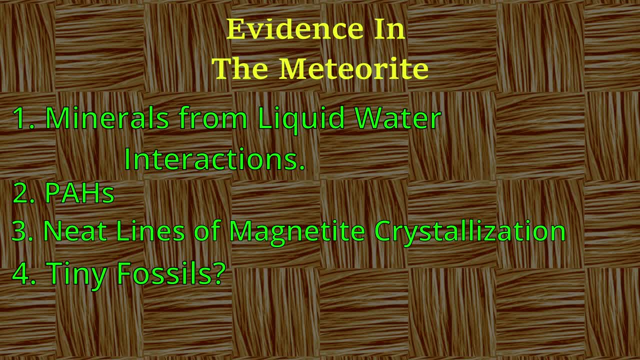 interactions of water. Two, there are PAHs, which just might be the remainders of bacteria that had died. Three, there are magnetites that are appearing in a way that they don't appear unless they're in actual bacteria which are producing them. 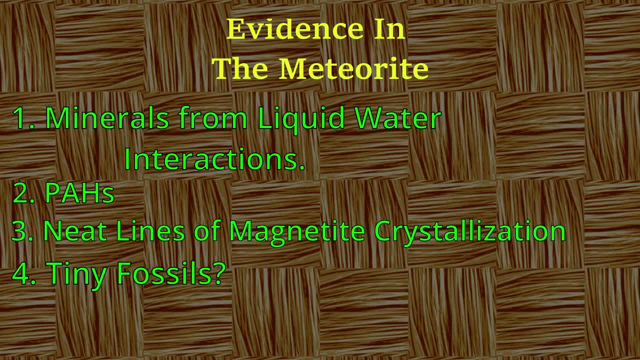 And lastly, it seems like we have little tiny, sausage-shaped fossils of actual fossil microbes. How do they appear? So the authors laid out all of this and they then closed with clarifying the thrust of their argument, And their argument is something like none of these observations are sufficient to prove. 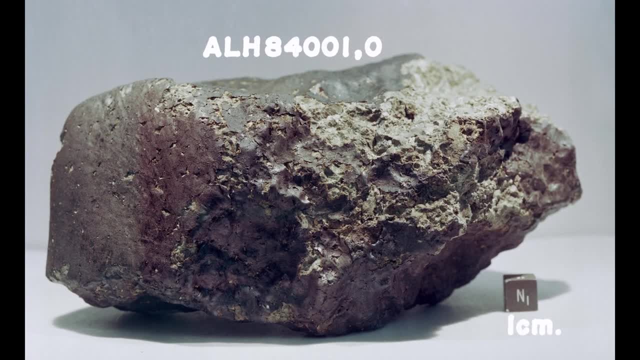 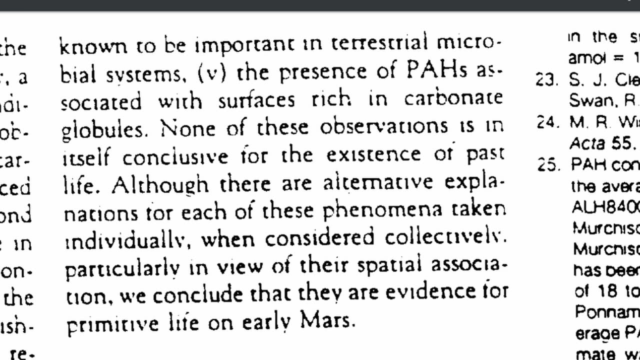 it, but look at the fact that we're finding all of this in one rock. That seems to be suggestive of life. To quote how they close their paper, none of these observations is in itself conclusive for the existence of past life, Although there are alternative explanations for each of these phenomena taken individually. 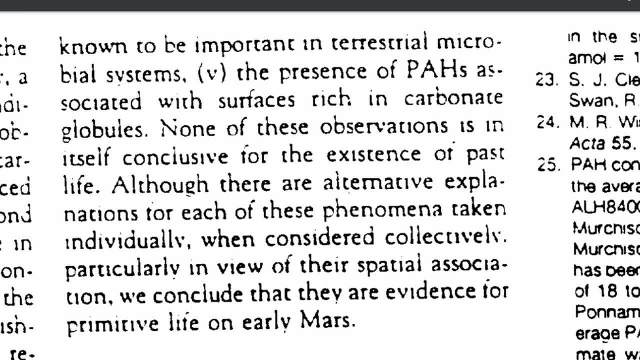 one of these observations is not conclusive for the existence of past life. When considered collectively, particularly in view of their spatial association, we conclude that they are evidence of permanent life on Mars. With this statement closing out their paper, a scientific frenzy ensued, and one by one, 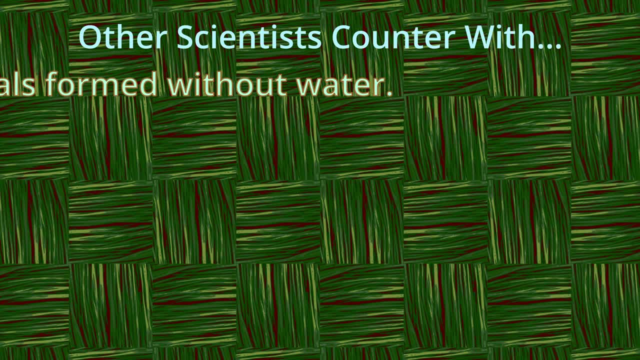 the lines of evidence were taken down, Those minerals that were supposedly created with liquid water could have been created without liquid water, and it's not like liquid water would be enough to prove the existence of life either way. These polycyclic aromatic hydrocarbons, PAHs, exist all over the place and, yes, that includes 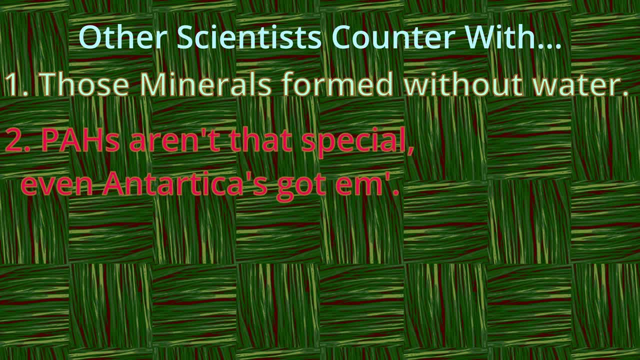 even the pristine Antarctic snow where the Martian meteorite had sat for 13,000 years. So maybe these PAHs are just from Earth and again, just like the liquid water. Even if these PAHs were from Mars, it wouldn't show anything in of itself either, because 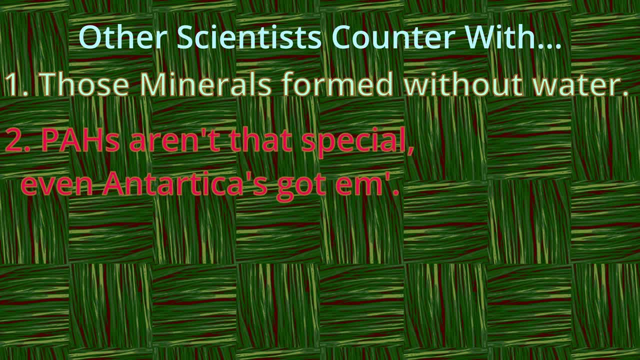 PAHs are found in interstellar dust and therefore they're going to come on asteroids and comets that flow to Mars and other planets. But now let's take a look at the two other, more suggestive pieces of evidence. How could these magnetite crystals have come to be? 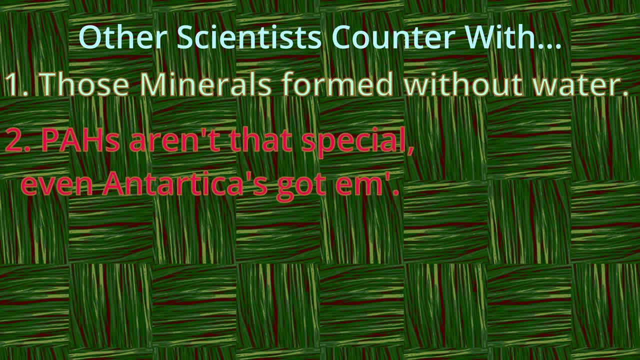 It's hard to say, And it seems that many scientists rejected this as significant evidence of life before there was actually sufficient explanation to explain how it might have come to be, and they were just saying, hey, this isn't enough. I'm sorry. 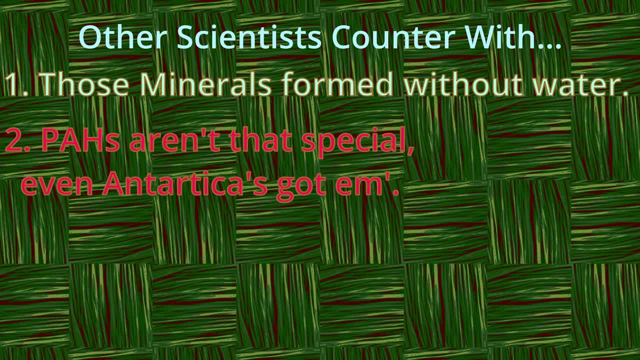 So there's a special type of crystal that we don't know how it might form in nature in this particular way, but it does form in nature. So maybe this is just a coincidence, But more recently some research has shown that they can be produced as shock minerals. 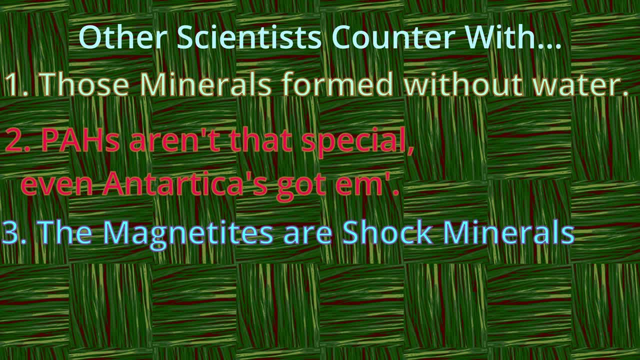 from extreme impacts that occur when asteroids hit the surface of a planet, in this case Mars. And another point raised by critics about these PAHs is that they can be produced as shock minerals from extreme impacts that occur when asteroids hit the surface of a planet. 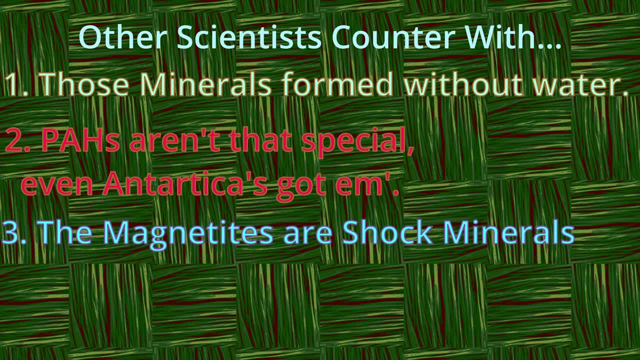 in this case Mars. And what's interesting about these magnetite crystals is that it doesn't quite make sense that these are what the people who say that this is evidence of life say they are, Because Mars has a much smaller metal core than Earth, so magnetic orienting, which some 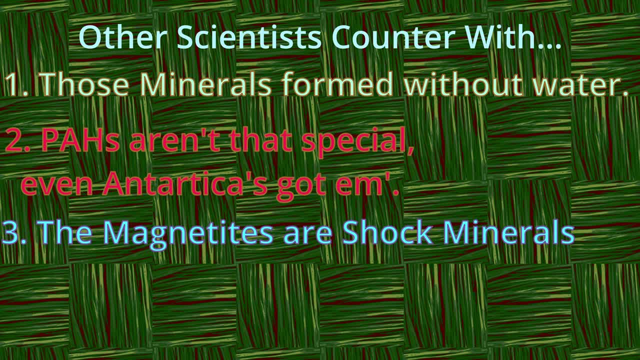 bacteria use on Earth with these magnetites. it's actually unclear that this would've been possible on Mars, given its small core. And finally, for the supposed fossil microbes themselves, many argue that they're pseudofossils created by natural means. 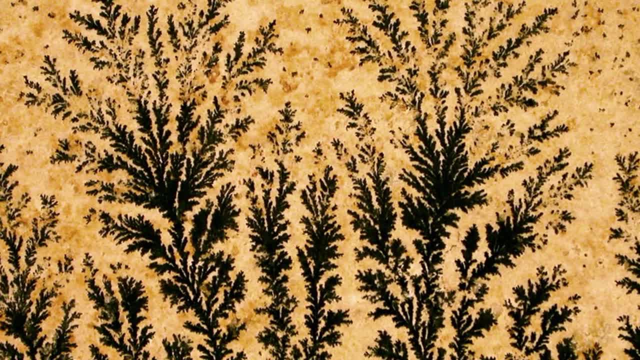 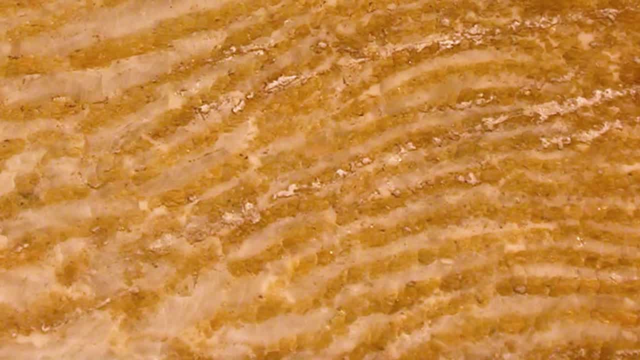 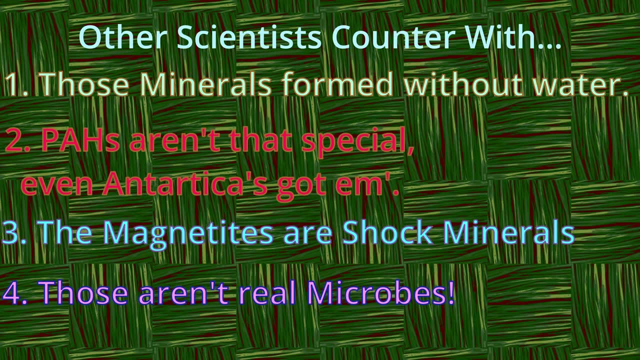 Take a look at this firm Nope, a crystal dendrite. It just looks like a fossil for her. And here take a look at some other great pictures of pseudofossils. Another point raised by critics about these supposed fossil microbes is that these fossil 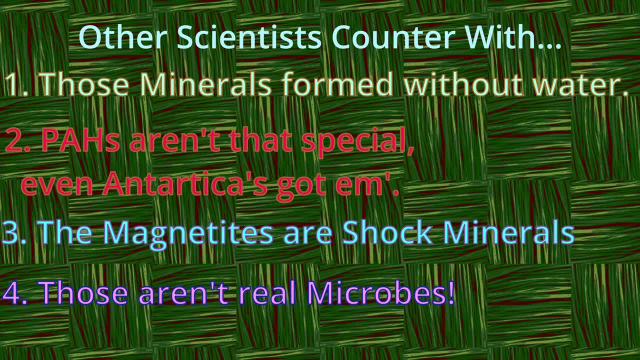 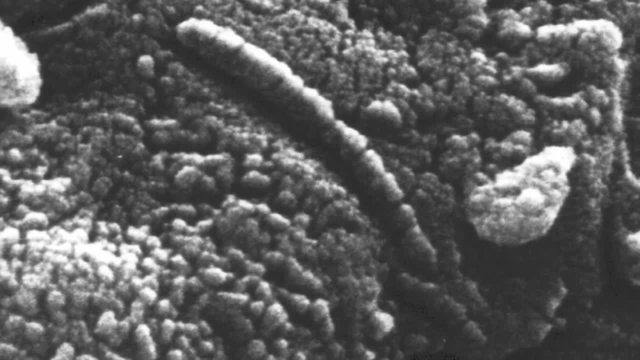 microbes are tiny in comparison to even the smallest life that we know of, and they would have been composed, based on their size, on only a few hundred biomolecules, which is much less than sufficient for the running of any known cell and, some argue, less sufficient. 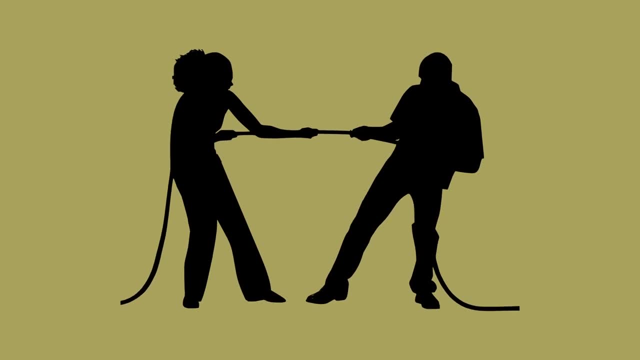 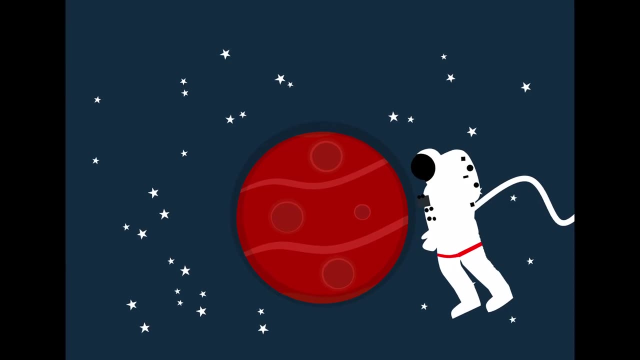 for the running of any cell period. Having gotten an idea of both sides now, wherever you land, whether you think the Martian meteorite shows signs of life or you don't, the possibility of life on Mars regardless of this meteorite. isn't incredibly far-fetched. Mars has plenty of chemical diversity, and it had liquid oceans for a while, and so it seems to at least have as much capacity as Earth has to produce life, or at least very close to the event. It's possible that we've seen more life in space, in the vacuum, than we've seen in the. 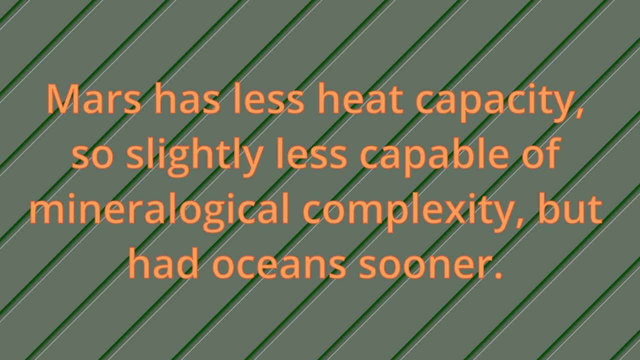 vacuum, and it's possible that we've seen more life in space than we've seen in the vacuum, But we don't know the exact amount that Earth has, because Mars doesn't in fact have as much long-term heat capacity as Earth, because it's smaller and therefore it cools faster. 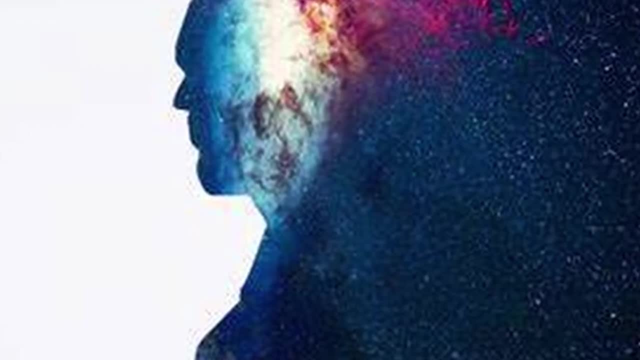 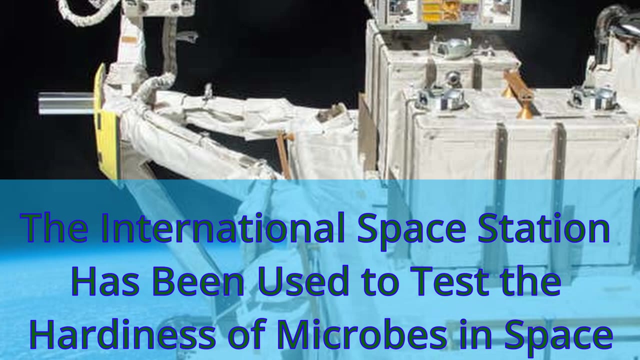 but it cooling faster also means that it got oceans sooner, so that means that fetal life might have gotten going earlier, so it could go both ways over here Once it leaves Mars. most life wouldn't survive in space. A human wouldn't survive more than a couple of seconds in the vacuum, but perhaps smaller. 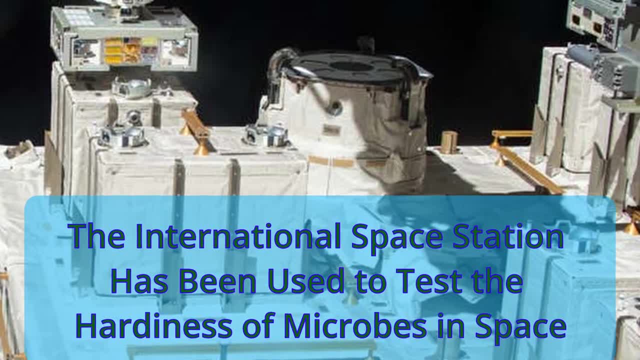 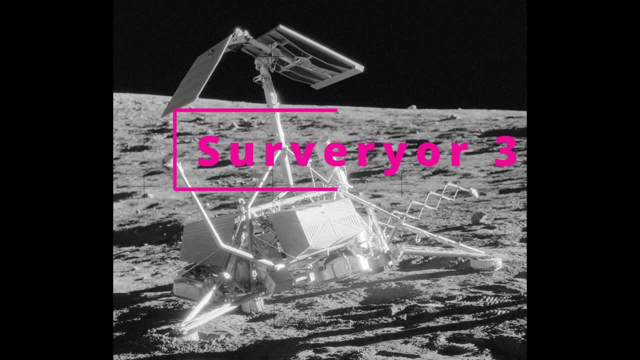 life actually could have. We know that groups of bacteria can last for up to 45 years in space, and it's possible that an individual bacteria survived for years in space as well. This is controversial but again really unresolved. In 1967, NASA sent a probe called Surveyor 3 to the Moon. 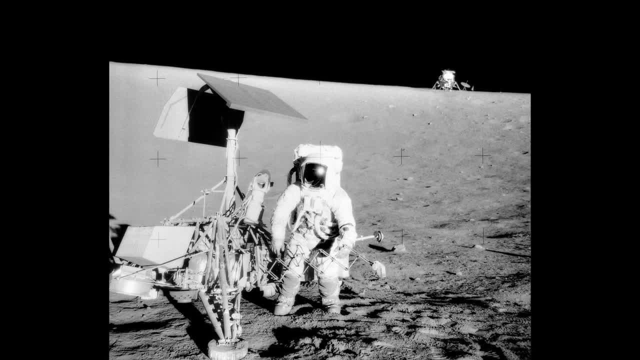 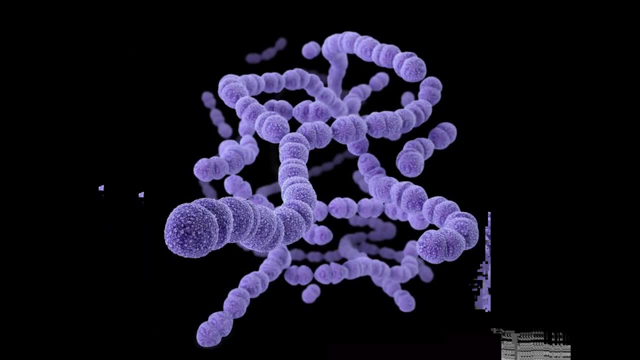 This was prior to actually sending actual humans to the Moon. So when the humans came, they removed the camera from Surveyor 3 and they brought it back to Earth, And here on Earth, when they analyzed it, they found some Streptococcus mitis. 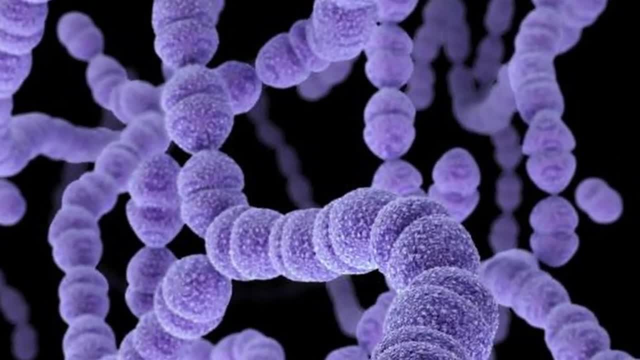 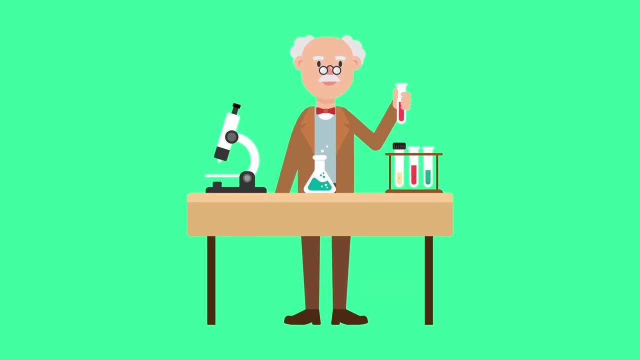 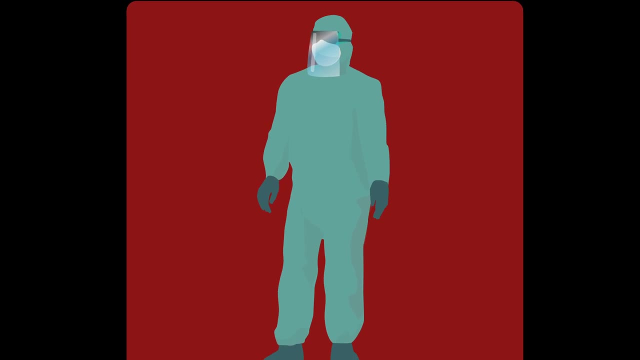 Where did this bacteria come from? Scientists at the time and some now argue that it came from Earth before it was sent, because it had proper procedures, in the views of these scientists, of preventing contamination on the way back, and it couldn't have come from the Moon. so it must have come from Earth. 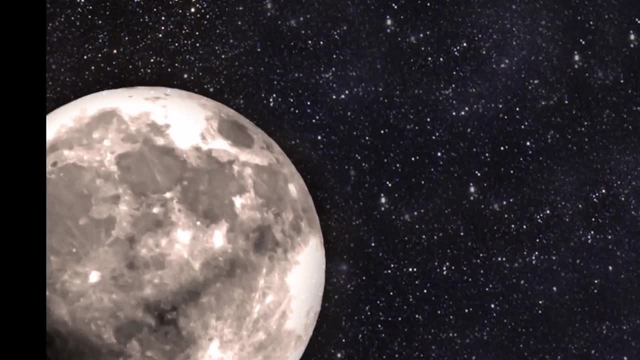 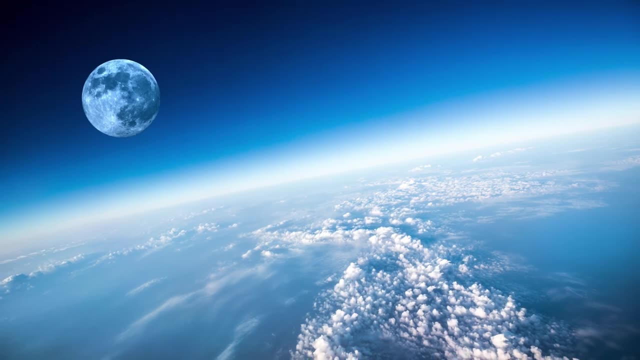 So that means it got on the camera on Earth. it then went up to the Moon and sat in a near vacuum with no nutrients or water, and exposed to ultraviolet radiation for two and a half years. and it then came back and lo and behold, this Streptococcus mitis was alive. 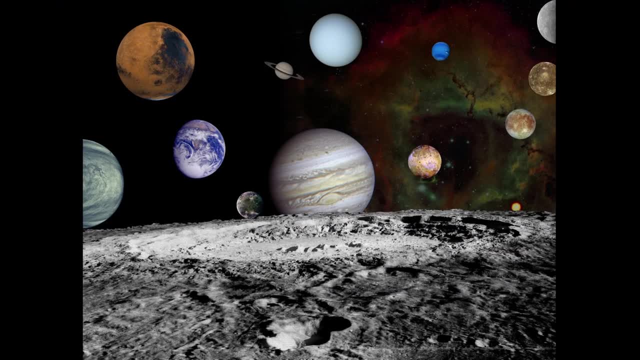 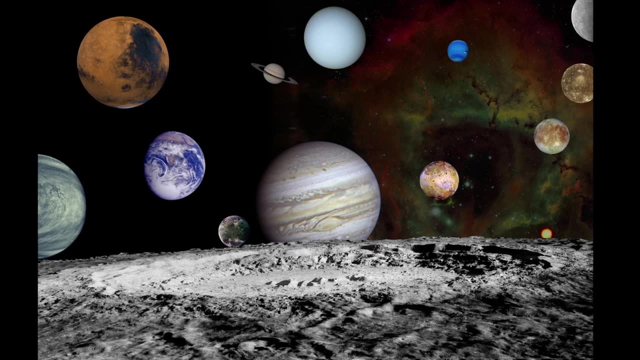 It was able to grow, it was able to replicate. so this would suggest that some basic forms of life could survive In the seemingly inhospitable home of space and still survived Now. some scientists since have argued that the bacteria, the Streptococcus mitis that 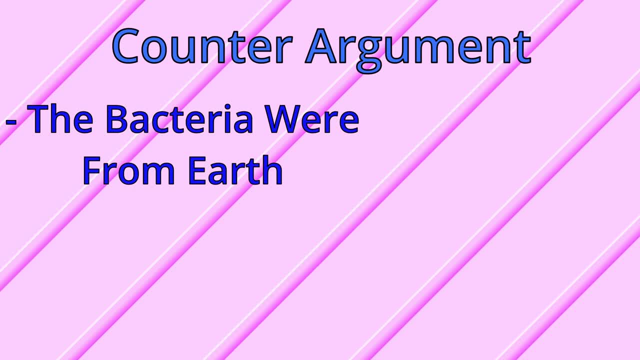 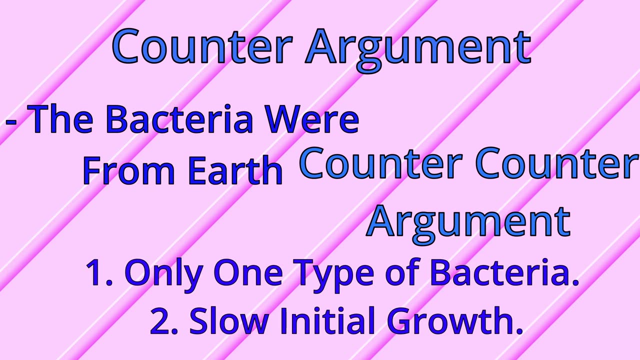 were found on the cameras were from when the camera came back and that the contamination procedures were insufficient. However, countervailing evidence to the idea that these bacteria had them sat there for two and a half years is that one only Streptococcus mitis were found and two the bacteria took. 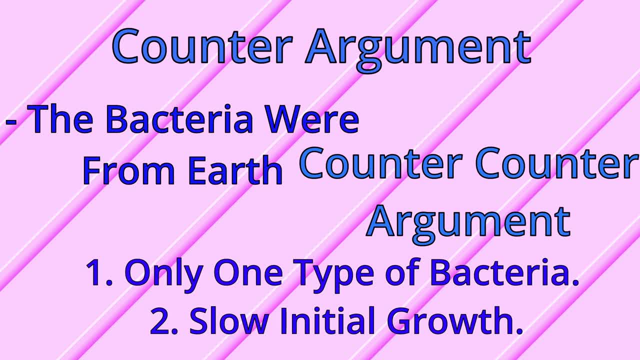 time to start growing, And if bacteria were a contamination from here on the way back, then they arguably should have been more varied and they should have grown faster, So they should have immediately started growing, instead of acting like starved and dormant bacteria. 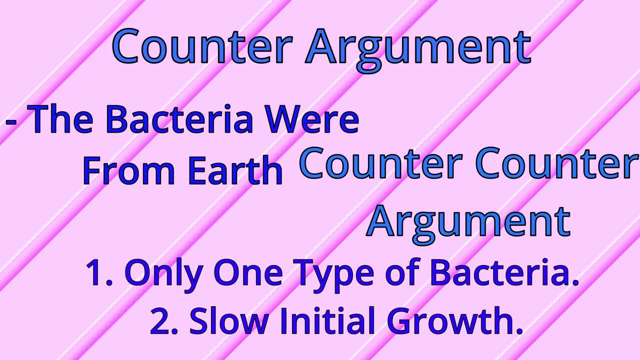 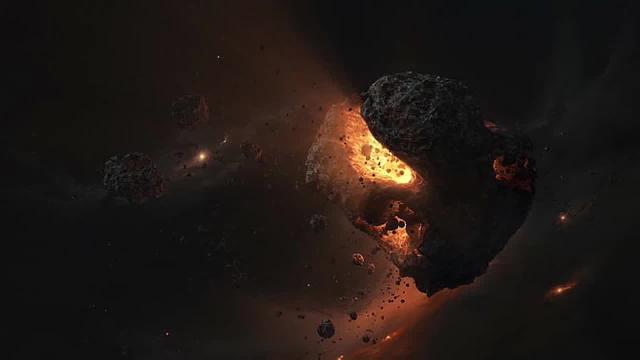 So that would demonstrate that bacteria might be able to survive, and we also have experiments that show that some bacteria can survive the kinds of extreme impacts they would experience crashing onto Earth. So the possibility of life arriving from space doesn't seem impossible. Now let's bring this whole conversation back to the historical question. 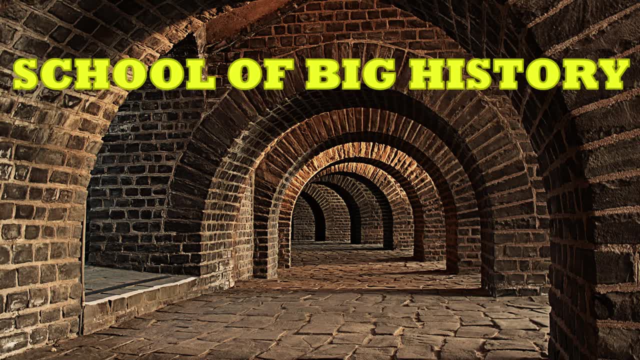 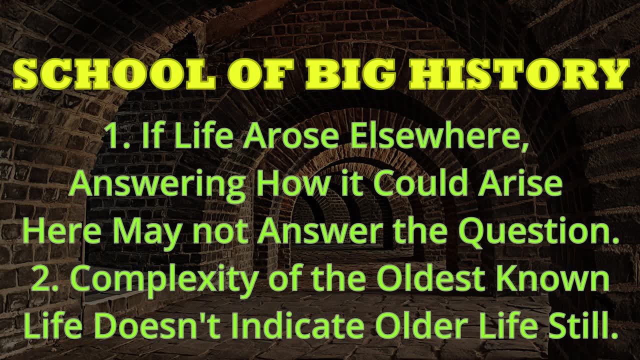 If life arose elsewhere and then came here, the question of how life arose is at least somewhat different than if it arose here, And also the earliest life on Earth that we know of can't be used to imply that life was here prior to them. 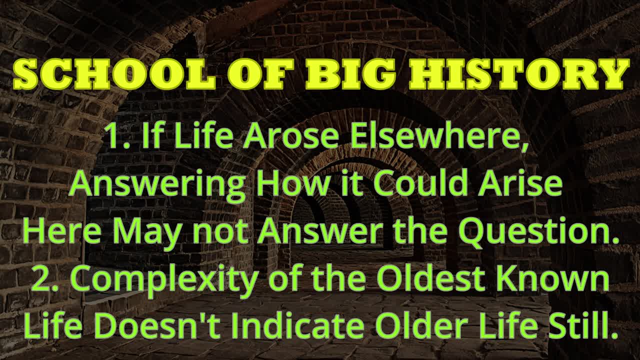 You can't look at the earliest life, for example, and say that because it's complicated, it must have been preceded by a lot more simple life here. After all, we'd have to know when and at how complicated a stage it arrived here as. 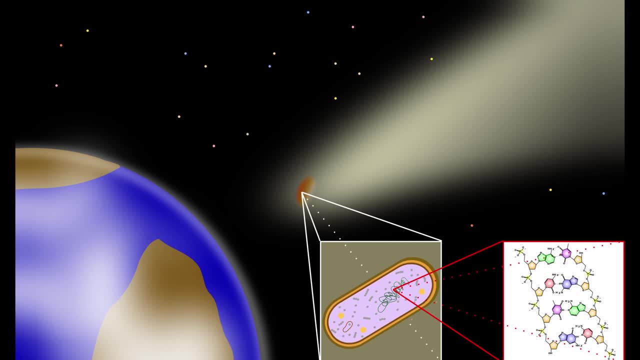 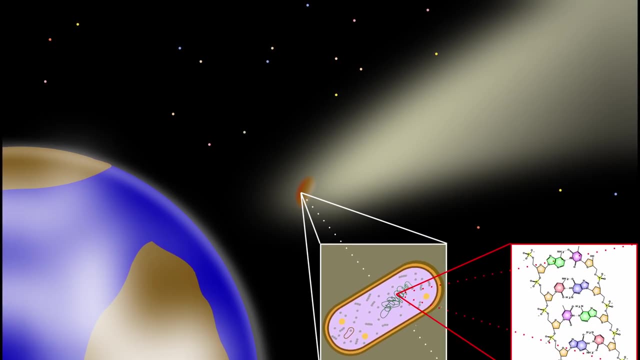 Despite this possibility of life having been complicated, we can't say that life arrived here prior to them. Much of the attention of origins of life scientists is on Earth, and estimates of the timing of the origin of life that you find in textbooks assume that life arose here. 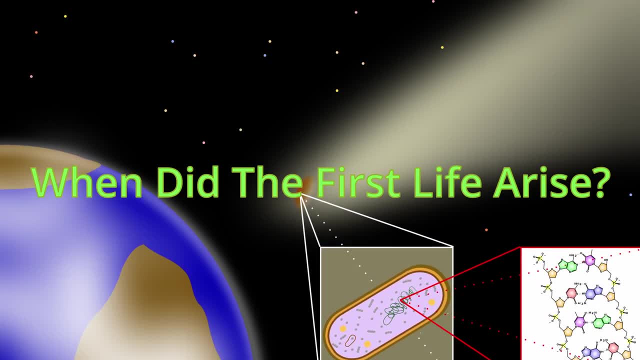 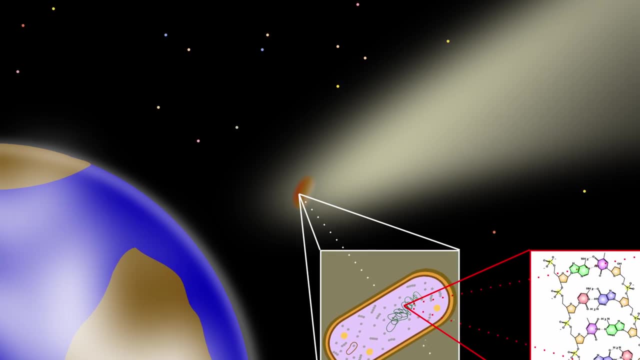 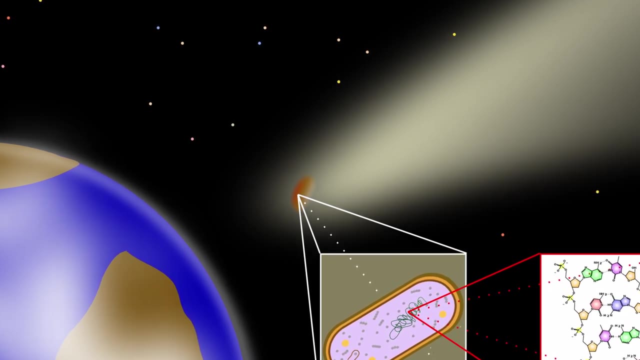 So for the coming video, we're going to assume right along with them and we're going to try to tag just when the earliest life arose here on Earth by taking a look at the oldest possible fossils. Thanks for watching. We'll see you next time. Bye. 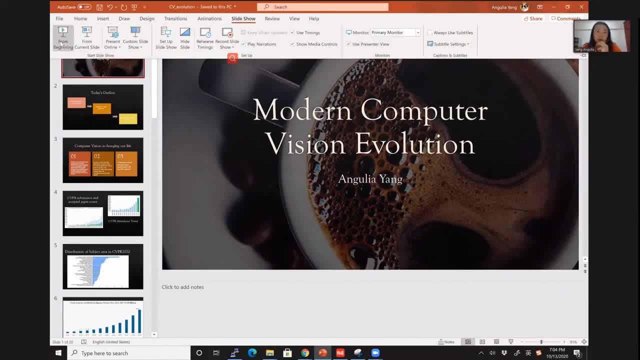 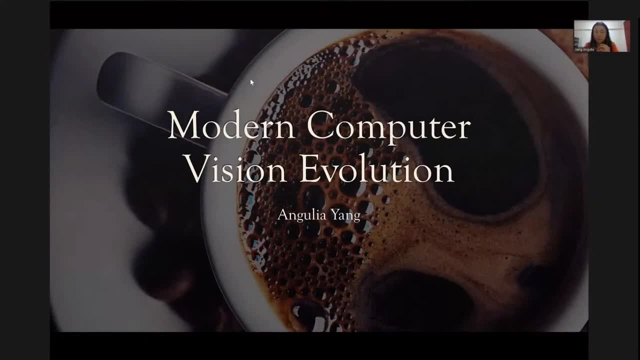 Everybody and again you know, good evening and welcome to our weekly sessions on AI ML. So, as we promised, we'll be bringing you a wide spectrum of topics. So today we are here with the Angulia Young for learning about computer vision.